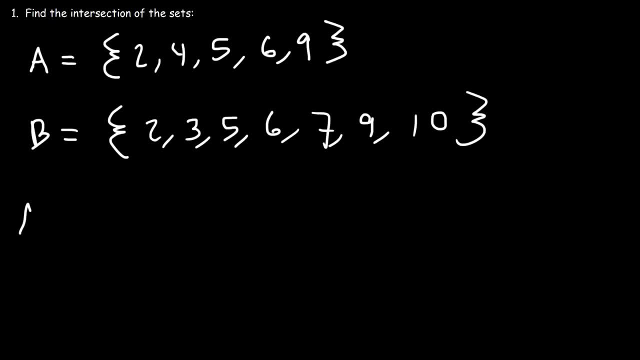 So what is the intersection of set A and B? How can we get the answer? To find the intersection, we need to find out which elements are common to both sets. So both sets contain a 2,, they contain a 5,, a 6, and also a 9.. 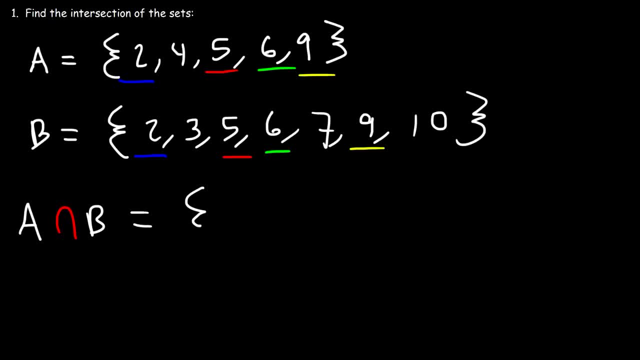 So, therefore, the intersection of sets A and B is 2, 3,- actually not 3,, but 2,, 5,, 6, and 9.. And that's it. So that's how you can find the intersection of two sets. 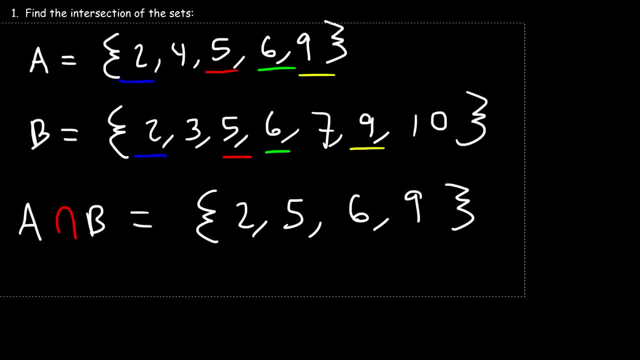 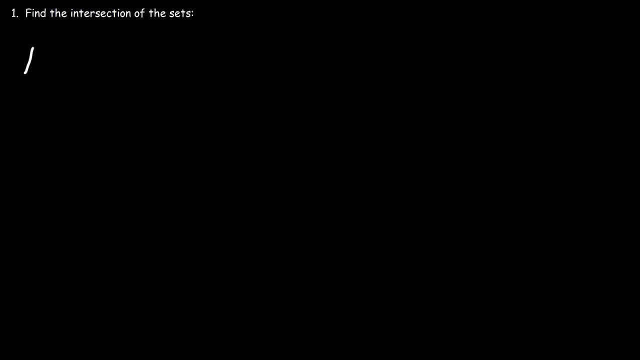 So now let's work on some more examples. You can pause the video and try this one if you want to. Let me use some different letters. So let's say this is set C and it contain the elements 3,, 4,, 6,, 7, and 10.. 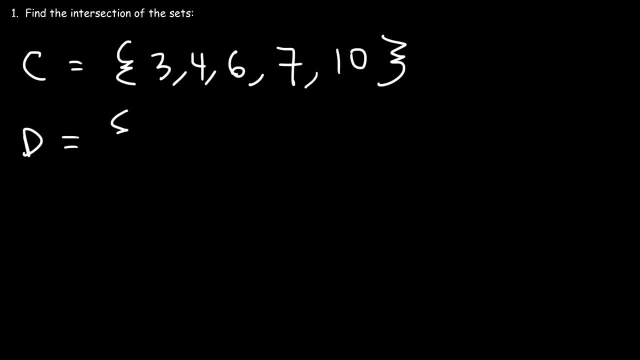 And also set D, which contain the elements 3,, 6,, 8, and 9.. So feel free to pause the video and determine the intersection of sets C and D. Go ahead and try it So which elements are common to both sets? 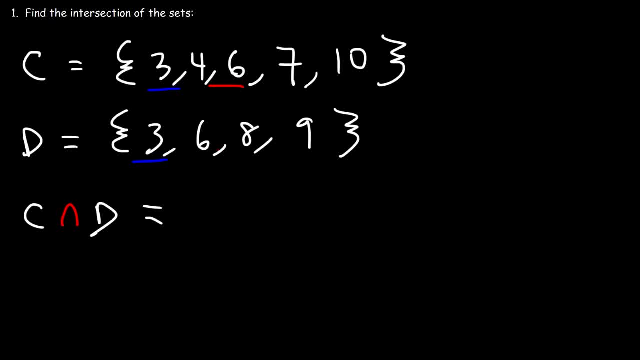 So 3 is common to both sets 6, and that's it. So for this particular example, it's only 3 and 6.. So that's the intersection of the two sets. So this is the answer. 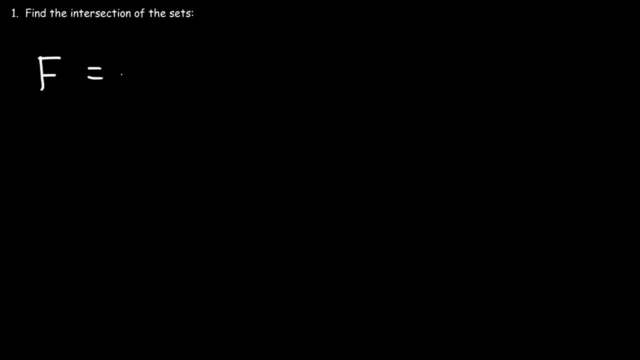 Let's try another example. Let's say Set F contains the elements A, B, C, D, F, G and J, And set G contains the elements A, C, G, H and K. So what is the intersection between sets F? 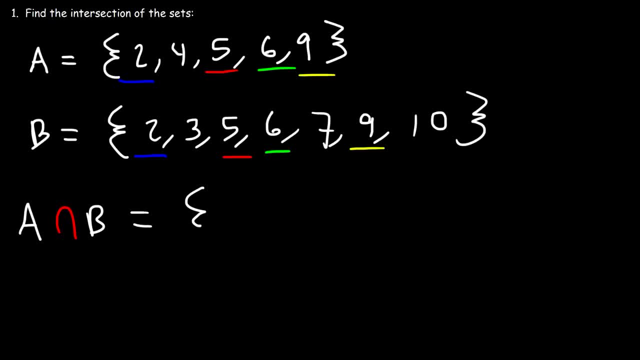 So, therefore, the intersection of sets A and B is 2, 3,- actually not 3,, but 2,, 5,, 6, and 9.. And that's it. So that's how you can find the intersection of two sets. 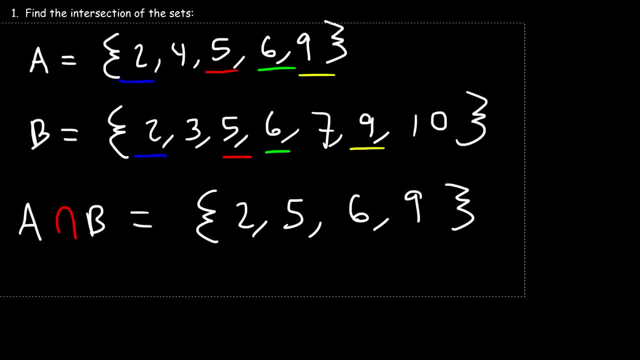 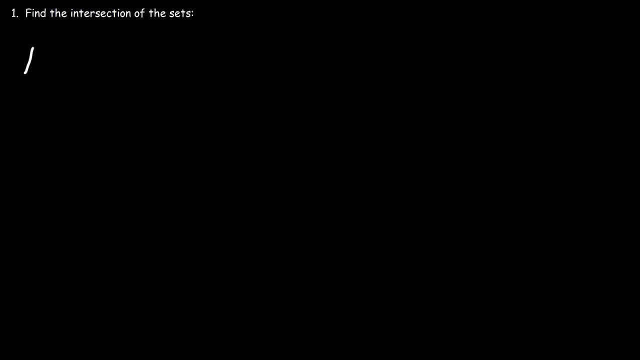 So now let's work on some more examples. You can pause the video and try this one if you want to. Let me use some different letters. So let's say this is set C and it contains the elements 3,, 4,, 6,, 7, and 10.. 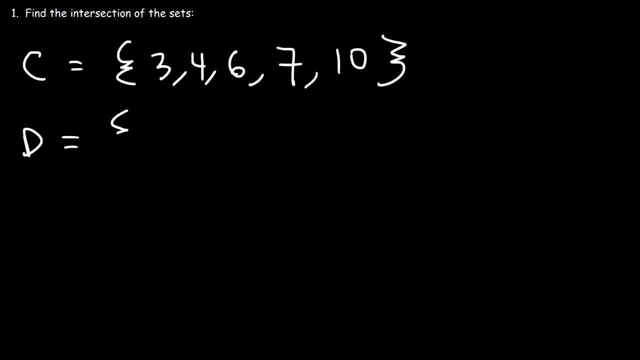 And also set D, which contain the elements 3,, 6,, 8, and 9.. So feel free to pause the video and determine the intersection of sets C and D. Go ahead and try it So which elements are common to both sets? 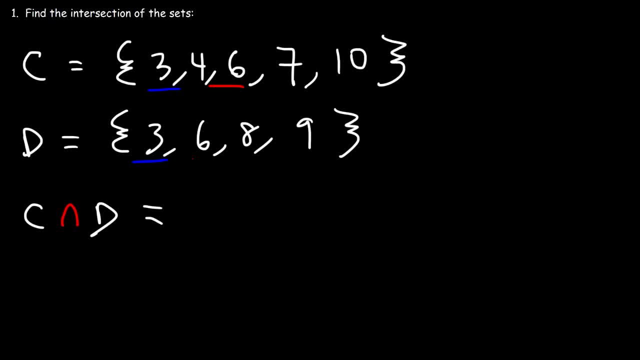 So 3 is common to both sets 6, and that's it. So for this particular example, it's only 3 and 6.. So that's the intersection of the two sets. So this is the answer. 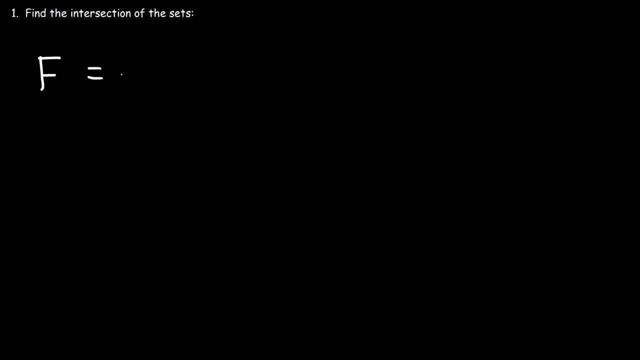 Let's try another example. Let's say Set F contains the elements A, B, C, D, F, G and J, And set G contains the elements A, C, G, H and K. So what is the intersection between sets F? 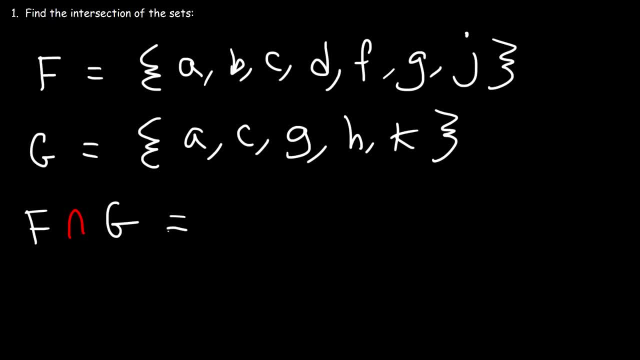 And G. So feel free to take a minute and try it. So let's see which elements are shared between both sets. So both sets contain element A, element C and G, And that is it. So the intersection of F and G is going to be A, C and G. 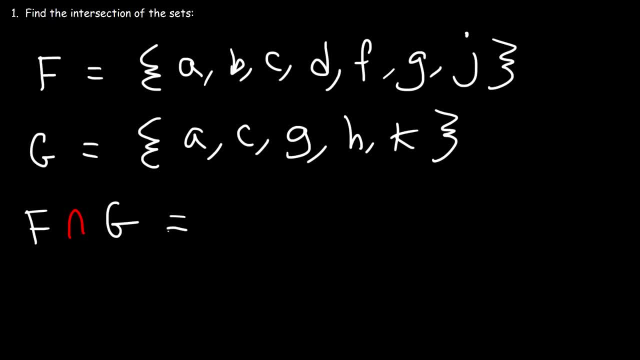 And G. So feel free to take a minute and try it. So let's see which elements are shared between both sets. So both sets contain element A, element C and G, And that is it. So the intersection of F and G is going to be A, C and G. 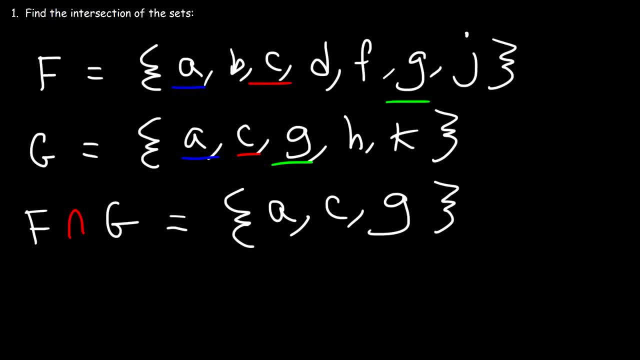 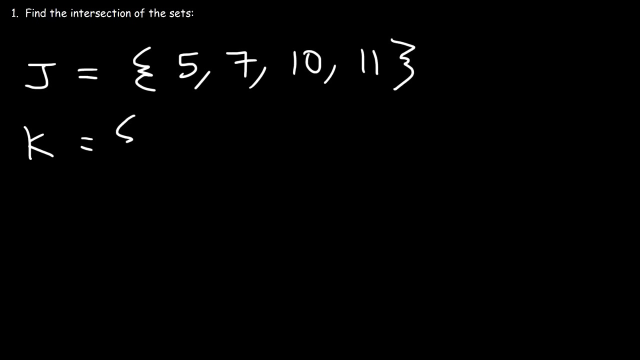 So, as you can see, finding the intersection is pretty straightforward. But now what about? Let's talk about this particular example. Let's say set J contains the elements 5,, 7,, 10, and 11.. And set K has the elements 2,, 4,, 8, and 13.. 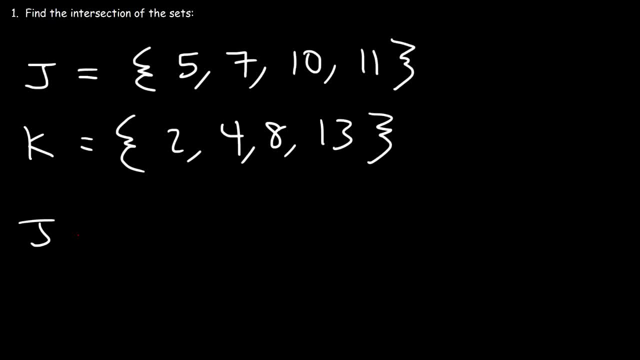 So what is the intersection of J? What is the intersection of J and 11?? What is the intersection of J and 11?? What is the intersection of J and K? Now notice that there is no common element shared between the two sets. 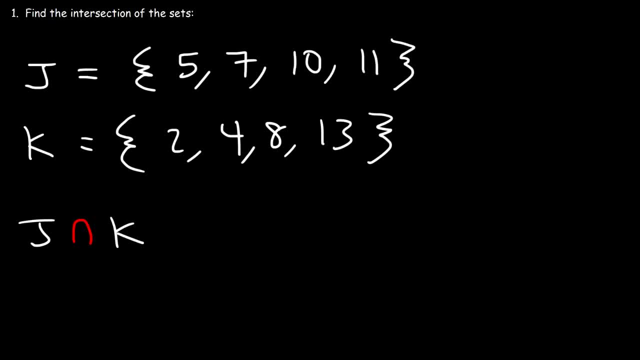 The elements in J are completely different from the elements in K. So in that case the intersection of J and K is going to be empty. There's going to be nothing inside. So if there's nothing inside, if you have an empty set, you have a null set. 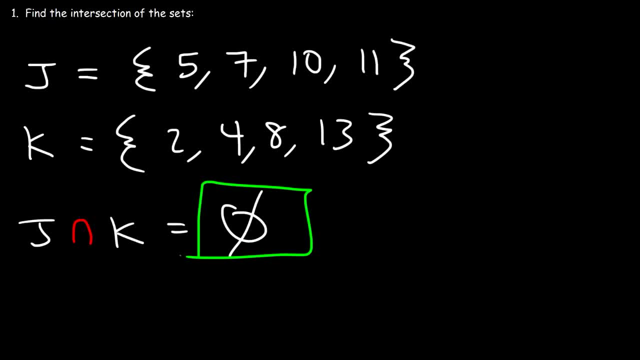 So this is the intersection of J and K. So this is the intersection of J and K. You have to use a Greek symbol, phi. Now let's say we have set R, which contains the numbers 3,, 4,, 7, and 10.. 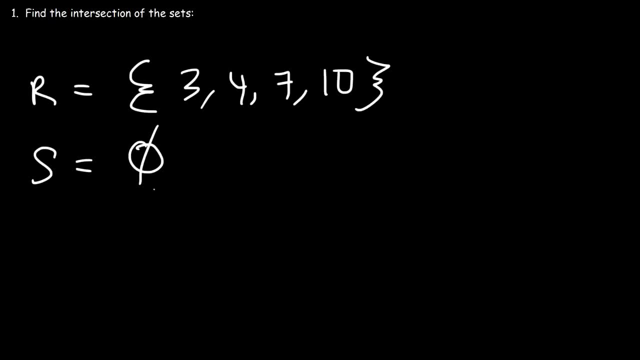 And set S, which is basically an empty set. What is the intersection of R and S? What is the intersection of R and S, The intersection of a set with numbers and an empty set? is going to be another empty set or a null set? 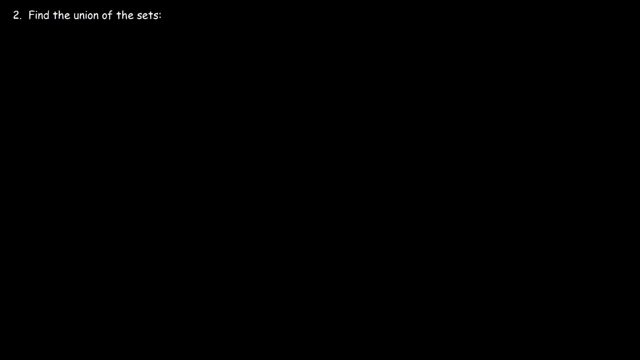 So that's it for this one. Now let's focus on a second type of problem that we need to talk about, And that is to find a union of two sets. So let's say that set A contains the elements 1 and 2.. 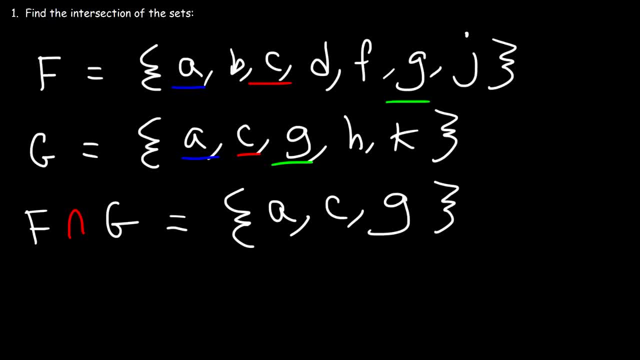 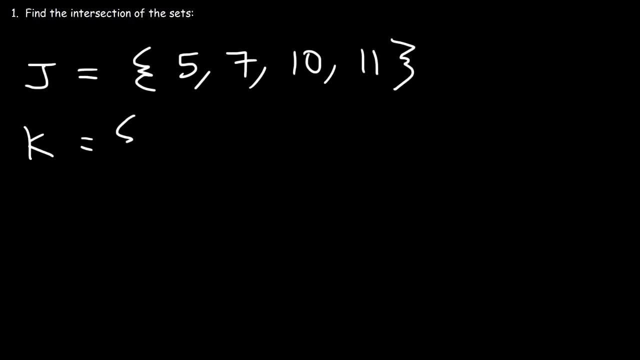 So, as you can see, finding the intersection is pretty straightforward. But now, what about This particular example? Let's say, set J contains the elements 5,, 7,, 10, and 11.. And set K has the elements 2,, 4,, 8, and 13.. 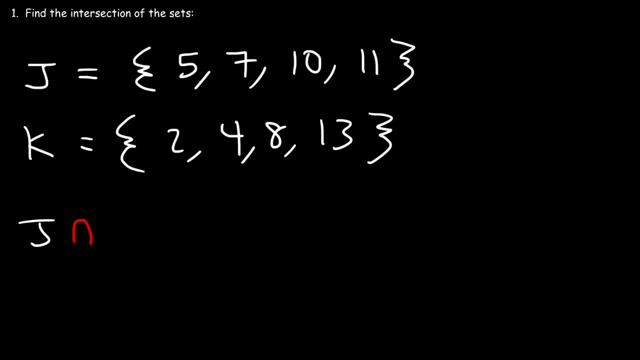 What is the intersection of J and K? Now notice that there is no common element shared between the two sets. The elements in J are completely different from the elements in K, So in that case, the intersection of J and K is going to be empty. 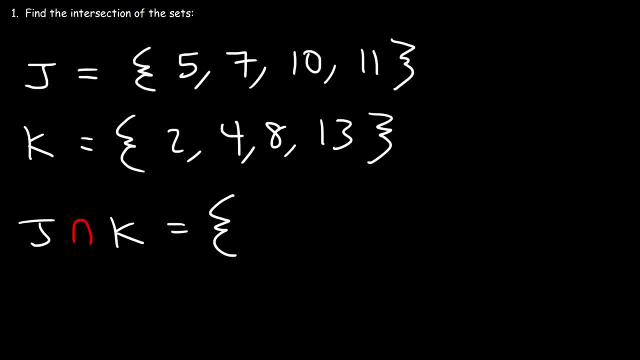 There's going to be nothing inside. So if there's nothing inside, if you have an empty set, you have a null set. So this is the intersection. You have to use a Greek symbol, phi. Now let's say we have set R, which contains the numbers 3,, 4,, 7, and 10.. 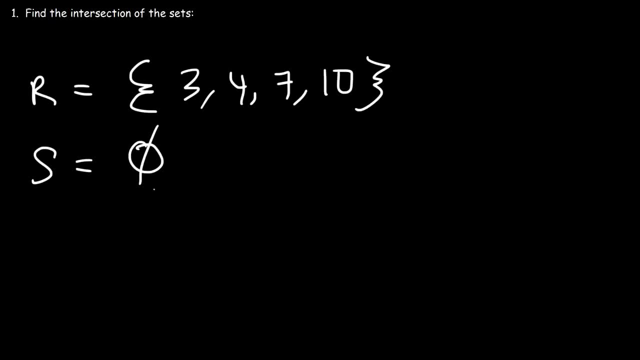 And set S, which is basically an empty set. What is the intersection of R and S? The intersection of a set with numbers and an empty set is going to be another empty set or a null set. So that's it for this one. 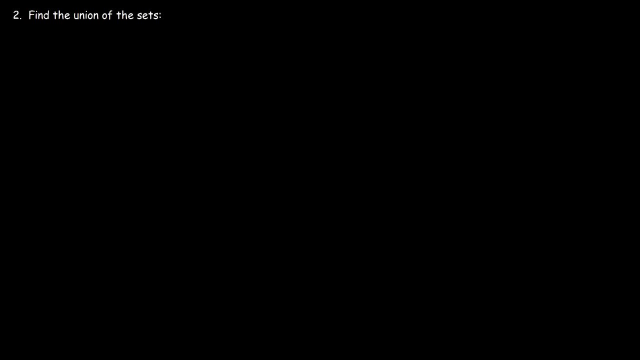 Now let's focus on a second type of problem that we need to talk about, And that is to find a union of two sets. So let's say that set A contains the elements 1 and 2.. 2,, 3, and 4.. 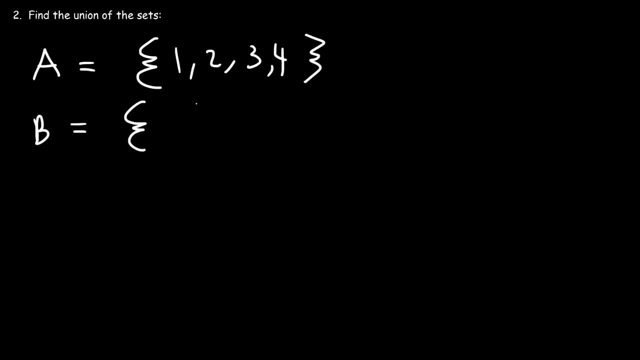 And set B contains the elements 3,, 4,, 5, and 6.. So what is the union of these two sets? When I think of union, I think of combining these into a larger set. Now notice that we do have some common numbers: 3 and 4.. 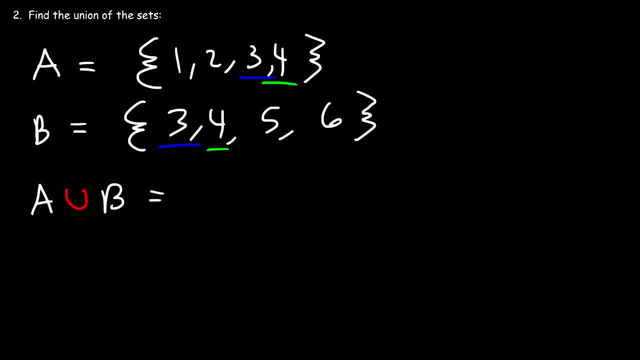 Now the union will contain everything in both sets But 3 and 4, we're not going to write it twice, only once. So the union of set A and B is going to be 1,, 2,, 3,, 4,, 5, and 6.. 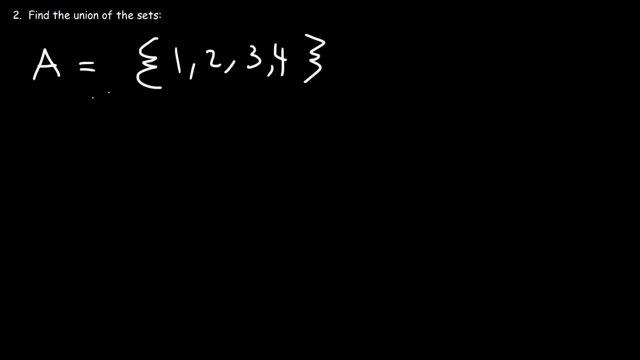 2,, 3, and 4.. And set B contains the elements 3,, 4,, 5, and 6.. So what is the union of these two sets? When I think of union, I think of combining these into a larger set. 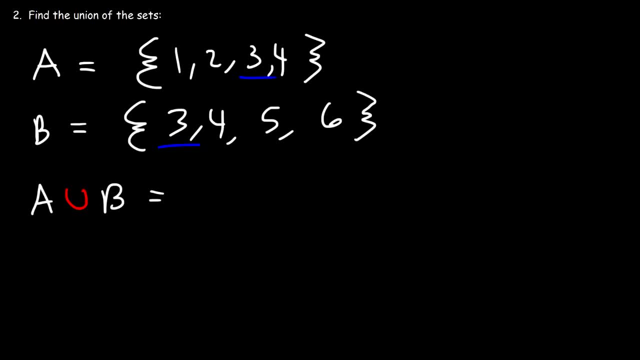 Now notice that we do have some common numbers: 3 and 4.. Now the union will contain everything in both sets But 3 and 4, we're not going to write it twice, only once. So the union of set A and B is going to be 1,, 2,, 3,, 4,, 5, and 6.. 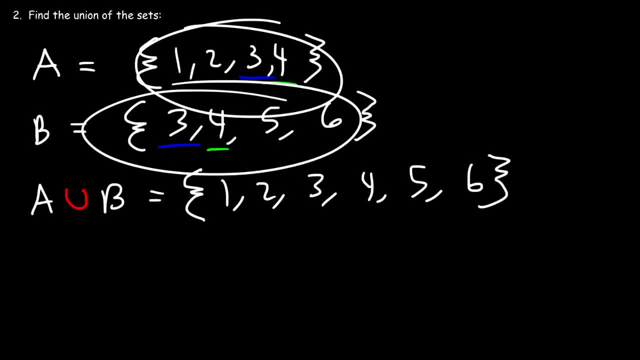 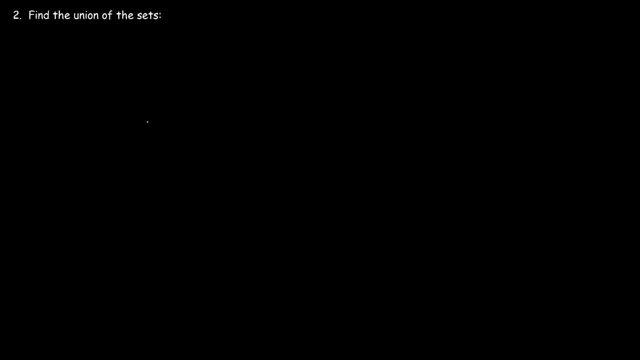 So we're going to write everything in both sets, but only write it once. So let's try some other examples. So let's say: set C is 3,, 5,, 9,, 11.. And set D is 2,, 3,, 6,, 8, and 12.. 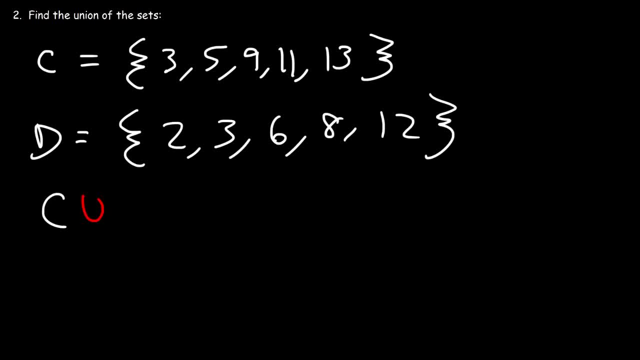 Go ahead and find the union between sets C and D. Go ahead and try that. So all we're going to do is just write all the numbers in C and D. So let's put it in ascending order. So we have a 2,, a 3, there's a 5.. 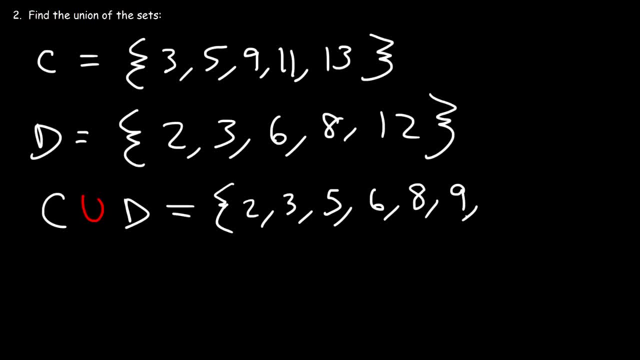 A 6,, there's no 7.. So we have an 8, a 9.. There's no 10,, but we have an 11,, 12, and 13.. And so that's it. So that's the union of those two sets. 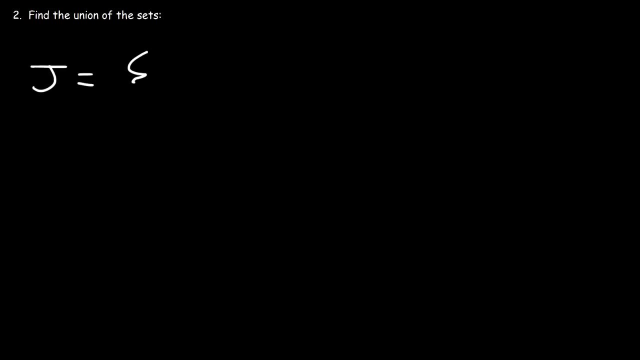 Here's another example. Let's say that set J contains the letters A, C, D, D and E and that set K contains the letters A, B, F, E and G. Go ahead and determine the union between J and K. 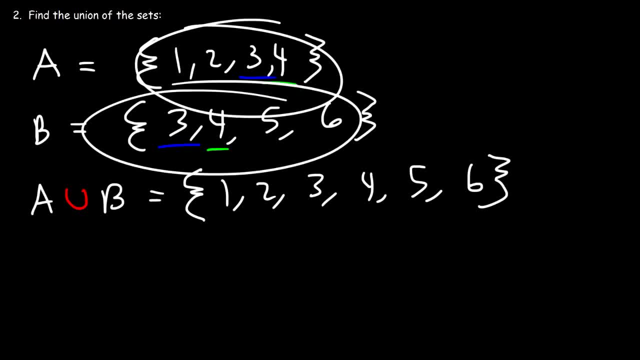 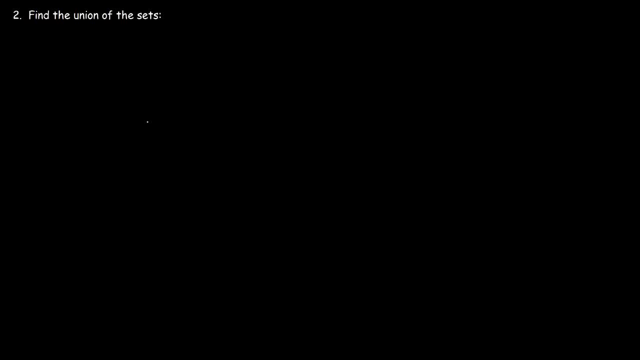 So we're going to write everything in both sets, but only write it once. So let's try some other examples. So let's say set C is 3,, 5,, 9,, 11, and 13.. 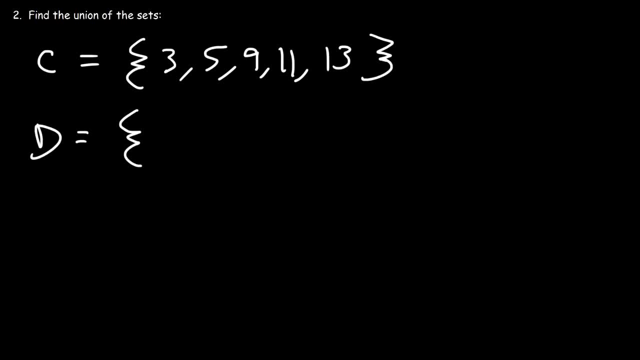 And set D is 2,, 3,, 6,, 8, and 12.. Go ahead and find a union between sets C and D. Go ahead and try that. So all we're going to do is just write all the numbers in C and D. 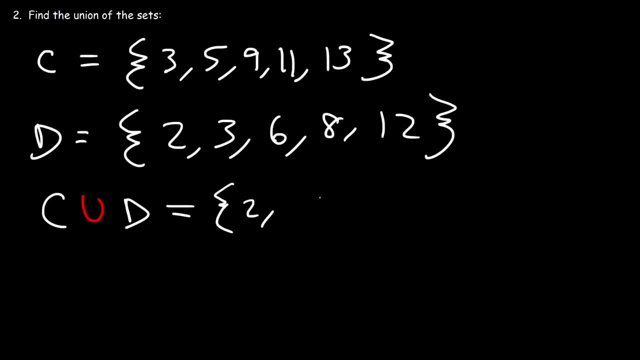 So let's put it in ascending order. So we have a 2,, a 3, there's a 5,, a 6,, there's no 7. So we have an 8, a 9,, there's no 10, but we have an 11,, 12, and 13.. 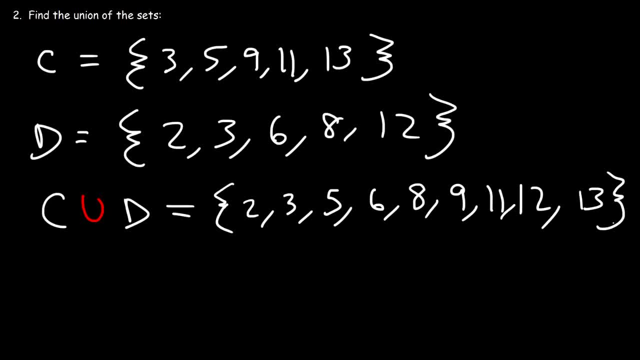 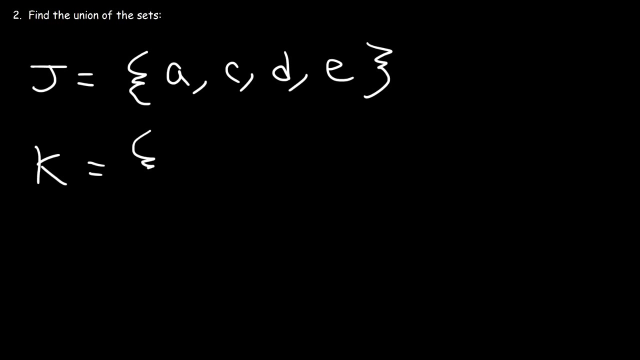 And so that's it, So that's the union of those two sets. Here's another example. Let's say that set J contains the letters A, C, D and E, And that set K contains the letters A, B, F, E and G. 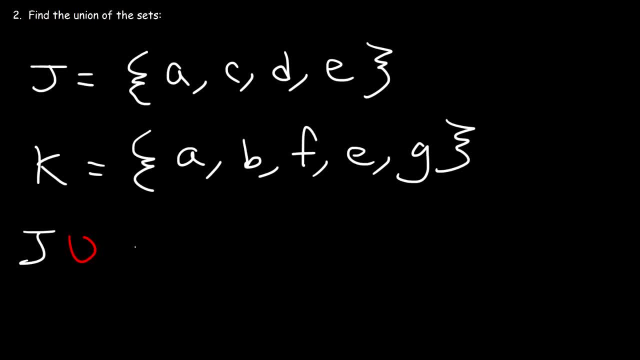 Go ahead and determine the union between J and K, So just like before. Oh, All we need to do is write all the letters. So we have an A, a, B, C, D, E, F and G. 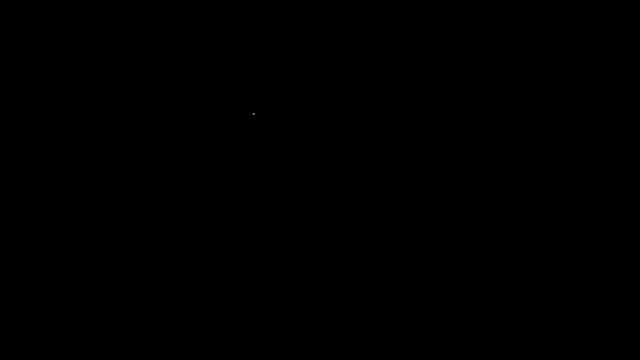 And that's it for that question. Let's say that set X contains the numbers 2,, 5,, 8,, 12.. And set Y, let's say, is an empty set. What is the union of a set with numbers and an empty set? 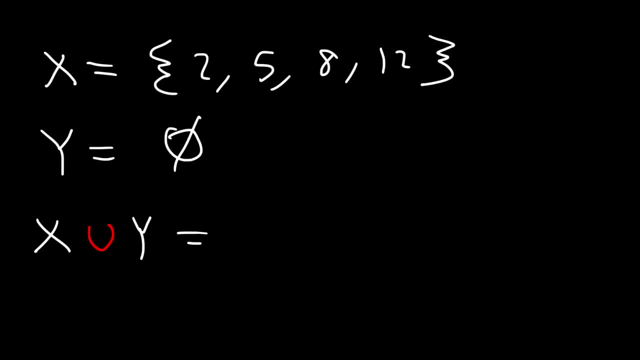 Well, the empty set. it's not going to add anything. It's like saying 15 plus 0.. That's going to be 15.. So, therefore, the union of set X with an empty set Y is going to be the same as set X. 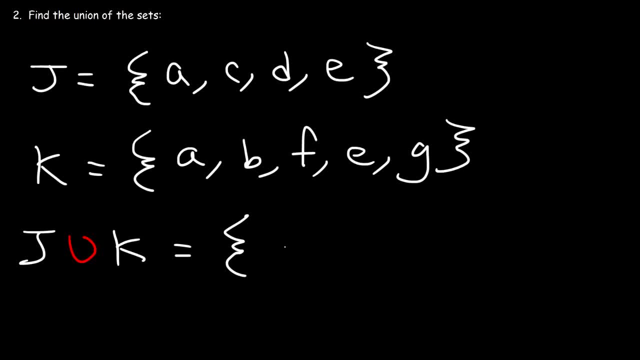 So, just like before, all we need to do is write all the letters. So we have an A, a, B, C, D, E, F and G, And that's it for that question. Let's say that set X contains the numbers 2,, 5,, 8,, 12.. 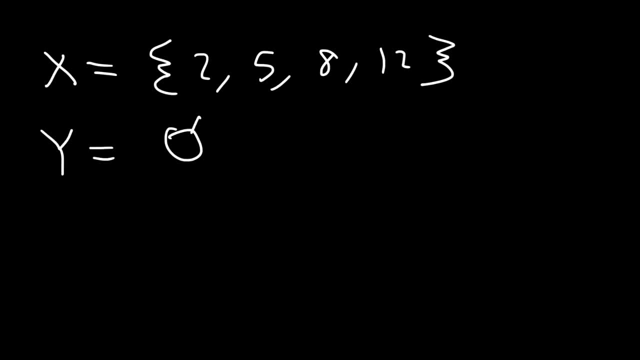 And set Y, let's say, is an empty set. What is the union of a set with numbers and an empty set? Well, the empty set is not going to add anything. It's like saying 15 plus 0. That's going to be 15.. 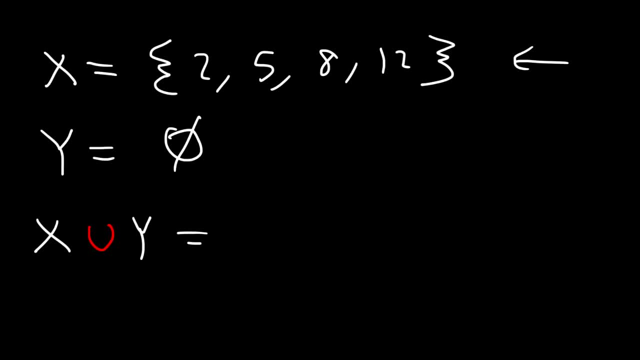 So, therefore, the union of set X with an empty set Y is going to be the same as set X. It's 2,, 5,, 8, and 12.. It's not going to change But the intersection of a set with something and a set with nothing. 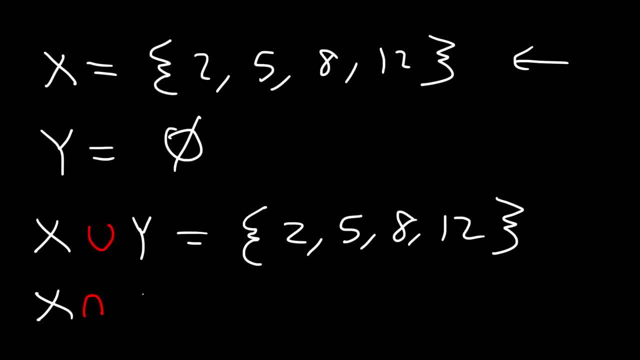 it's going to be an empty set. So just something to keep in mind. Now here's a question for you. Let's say, if set A contains the numbers 3,, 4,, 5, and 7.. 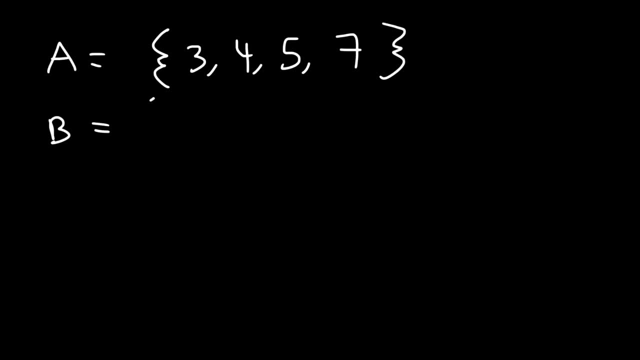 And set B contains the numbers 2,, 4,, 5, and 8.. How can you determine the intersection of A and B and the union of A and B and represent the results using a Venn diagram? So circle A and circle B. 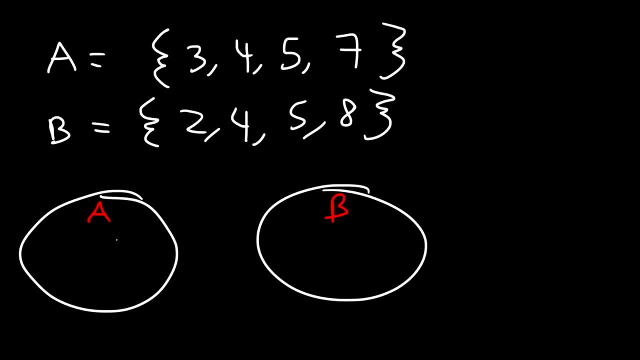 In its separated form. Set A contains the numbers 3,, 4,, 5, and 7.. And B contains the numbers 2,, 4,, 5, and 8.. Now the intersection of these two. I'm running out of space here. 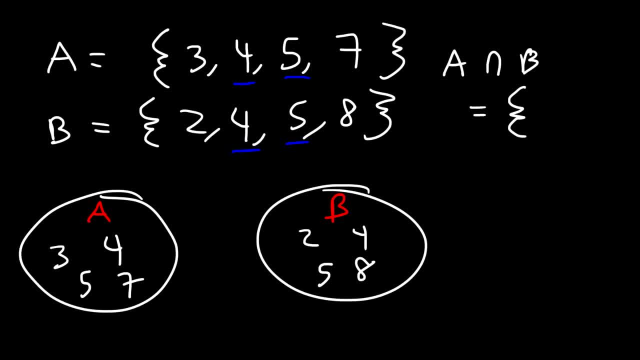 is 4 and 5.. 4 and 5 are found in both, But to represent that using Venn diagrams, what we need to do is put the two circles together And draw it this way. So this is set A and set B. 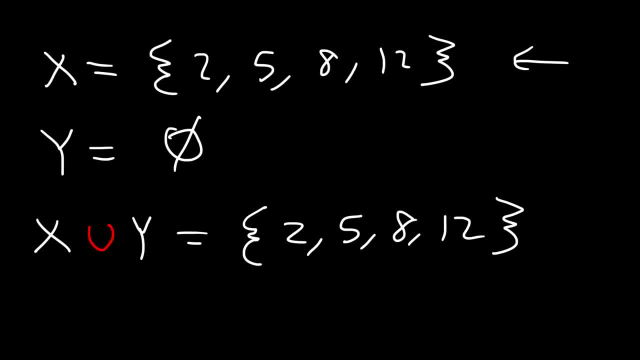 It's 2,, 5,, 8, and 12.. It's not going to change But the intersection of a set with something and a set with nothing. it's going to be an empty set, So just something to keep in mind. 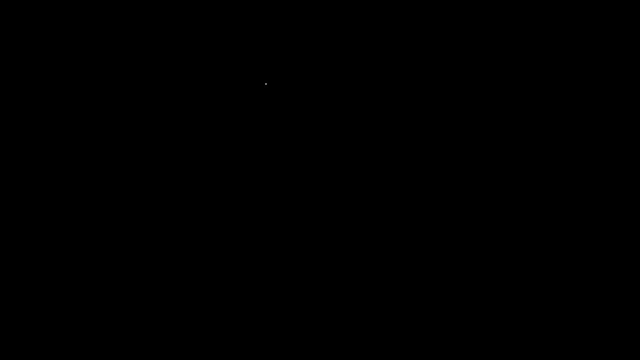 Now here's a question for you. Let's say if set A contains the numbers 3,, 4,, 5, and 7. And set B contains the numbers 2,, 4,, 5, and 8. How can you determine the intersection of A and B? 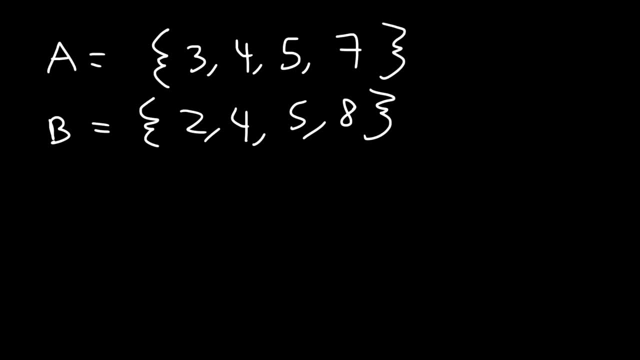 And represent the results using a Venn diagram. So circle A and circle B in its separated form, Set A contains the numbers 3,, 4,, 5, and 7.. And B contains the numbers 2,, 4,, 5, and 8.. 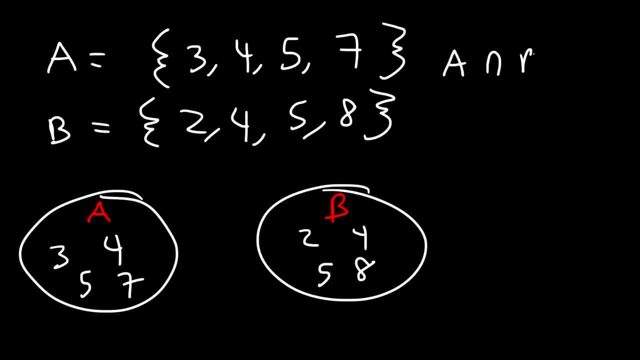 Now the intersection of these two- I'm running out of space here- Is 4 and 5.. 4 and 5 are found in both, But to represent that using Venn diagrams, what we need to do is put the two circles together. 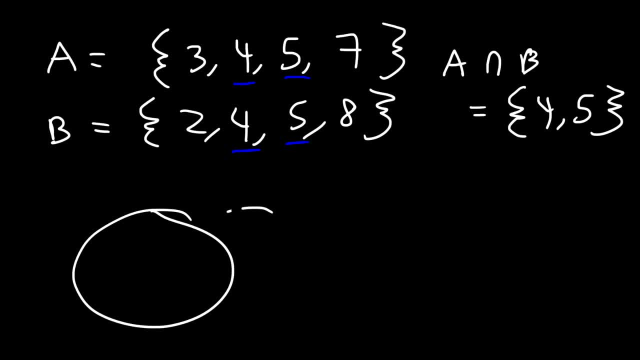 And draw it this way. So this is set A and set B. So in the middle is the intersection of A and B, And this is the intersection of A and B. So in the middle is the intersection of A and B. 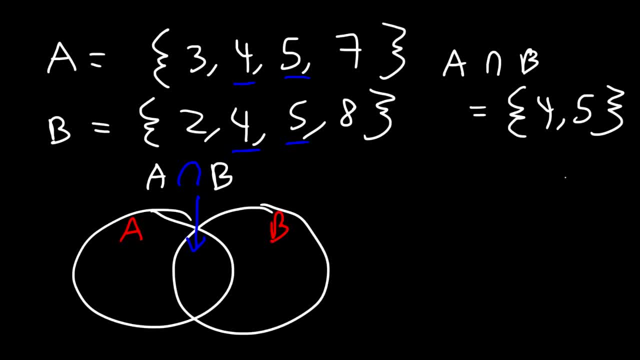 B, which contains these elements: four and five. now a also contains three and seven, and B also contains two and eight, but four and five is common to a and B, so we put that middle. now the union of these two sets is basically everything. it contains the numbers two, three, four, five, seven and eight, and I'm running out of. 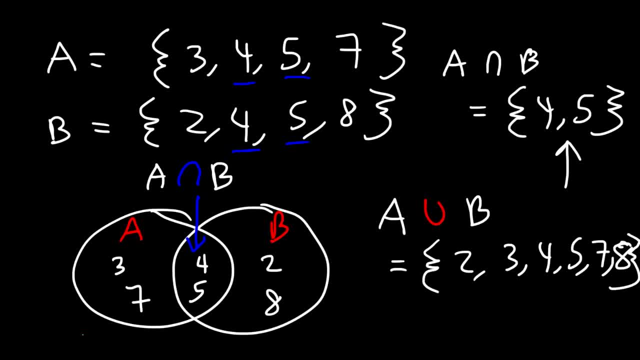 space. so this entire system with the two circles represents the union of a and B because it contains all the numbers two, three, four, five, seven and eight. but the intersection is limited by this region here because it only contains the elements common to both sets. so hopefully this helps you to see the relationship between intersection of. 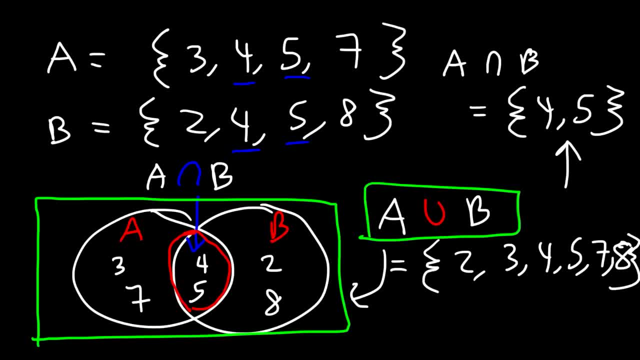 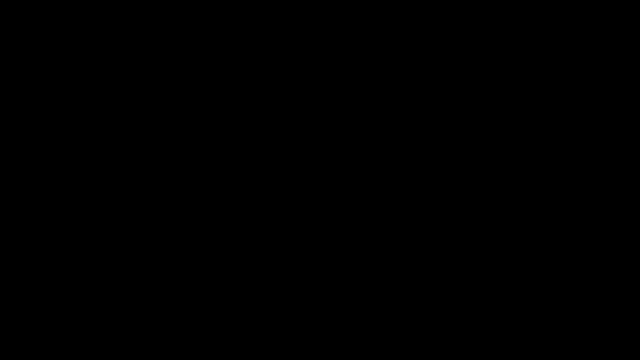 sets and union of sets as it relates to Venn diagrams. so that's it for this video. thanks for watching and have a good day you. 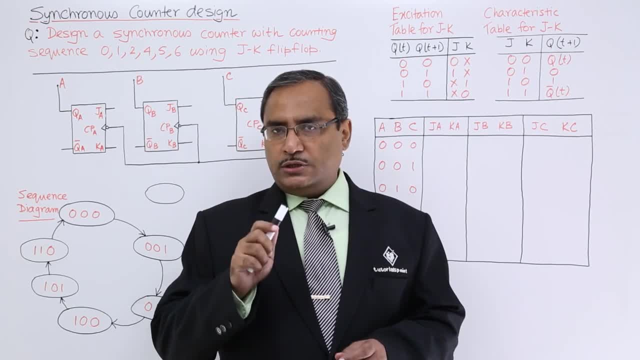 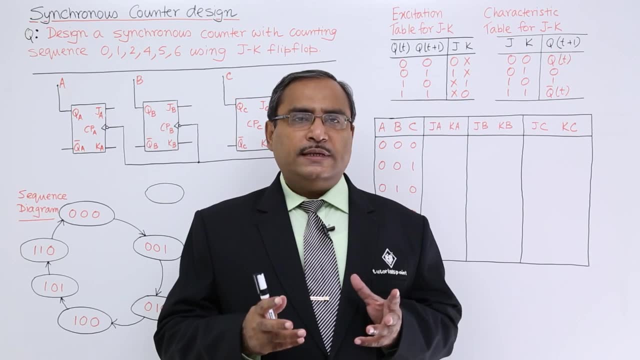 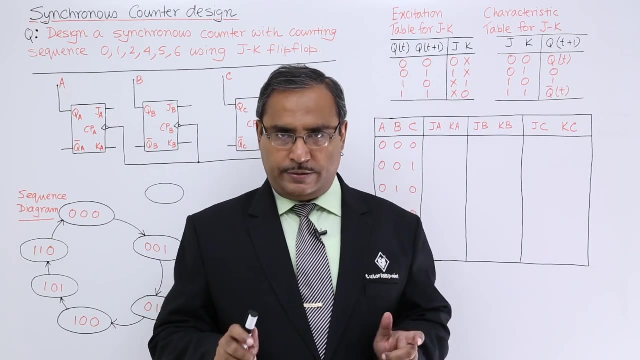 Synchronous counter design. In this session we shall solve one problem on synchronous counter design and we shall tell you that how all the problems in synchronous counter design can be solved and what is the general rules and steps to be maintained. So here is one. 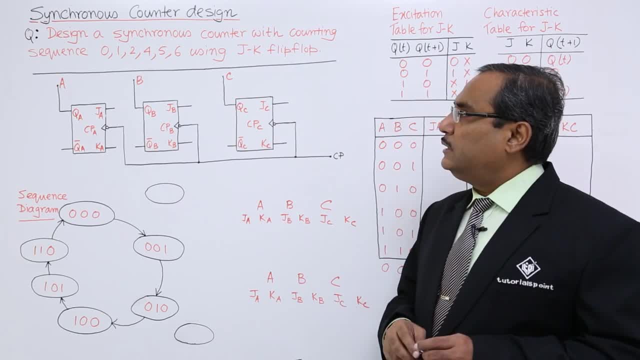 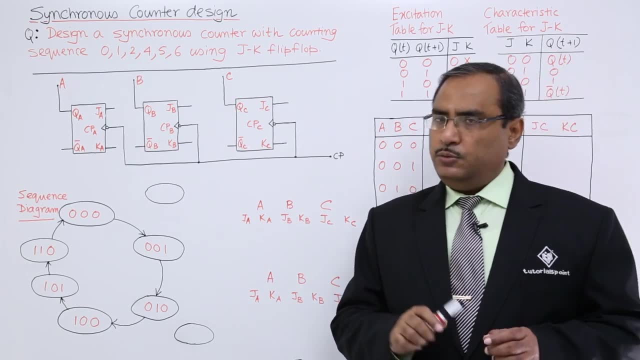 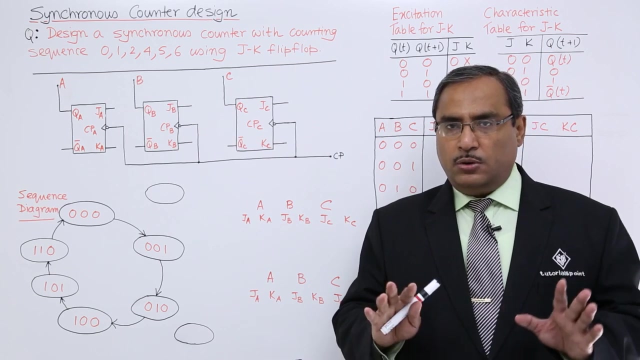 question for us: Design a synchronous counter with counting sequence 0,, 1,, 2,, 4,, 5, 6, using JK 5th block. So here we are supposed to note that whether it is synchronous or asynchronous, in the question it is mentioned as synchronous. We have got that point. The 5th block name. 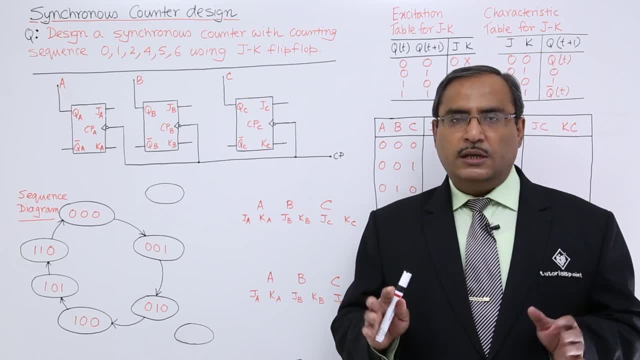 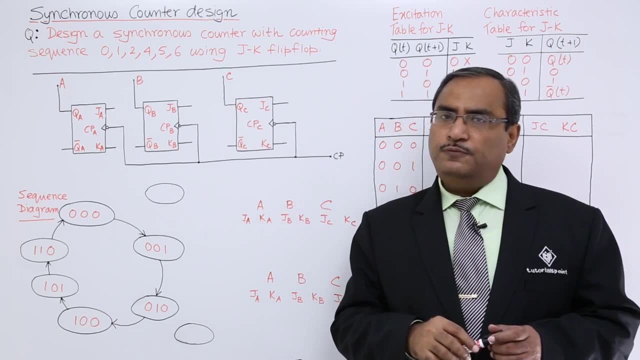 is mentioned. Yes, JK 5th block. So there is no other options. Otherwise, we can take other 5th blocks also. So now next point is that: what is the counting sequence? 0,, 1,, 2,, 4,, 5,, 6.. What is the maximum number here? 6.. So how many bits will be required to represent? 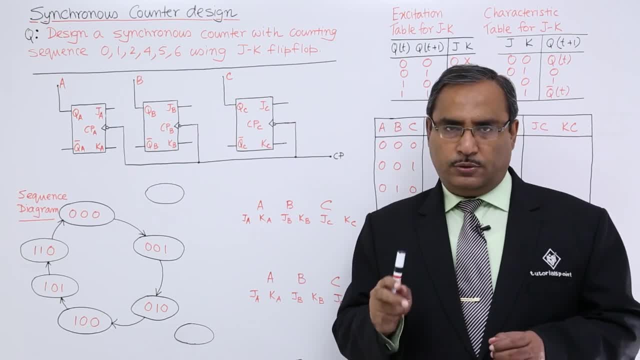 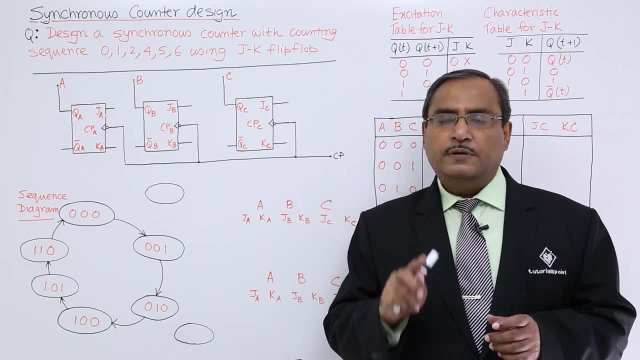 6? 3 bits. What are they? 1, 1, 0.. So that will represent 6.. So that means this particular counter design will require 3 number of JK 5th blocks. So that is why I have drawn this JK 5th blocks.